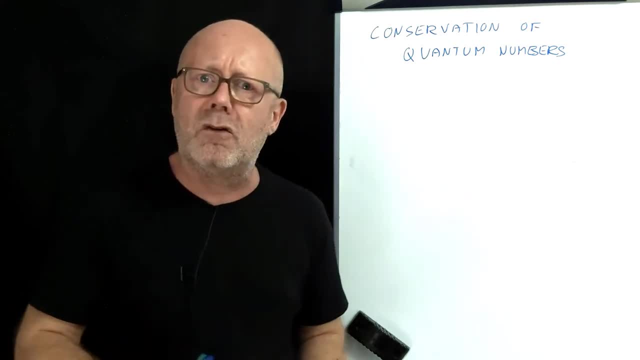 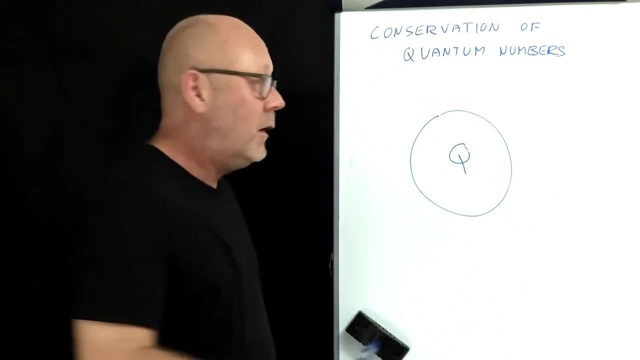 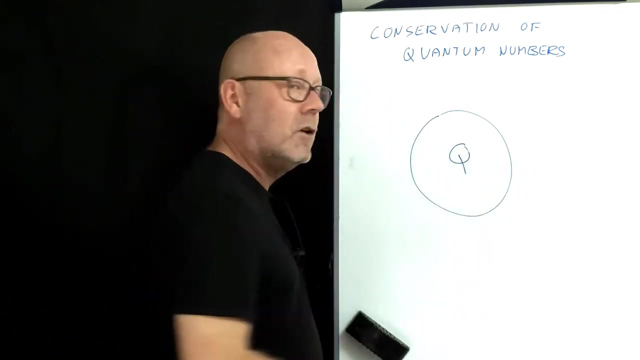 conserved needs to stay the same. Say, let's use conservation of charge. If I have a universe with a certain amount of charge Q in it and this universe is isolated from the rest, the charge Q will remain the same. Whatever happens inside the universe, Q will always stay the same. We can use 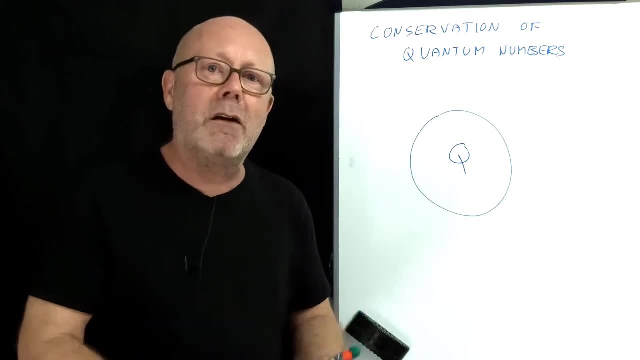 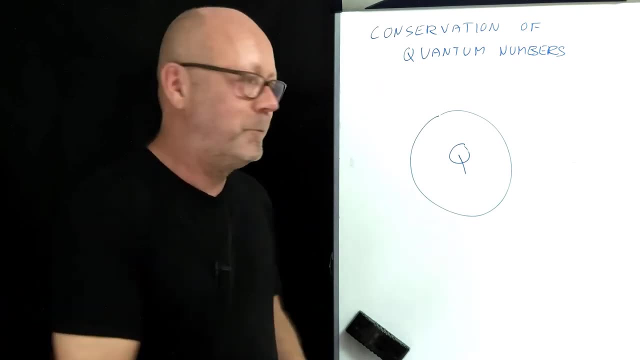 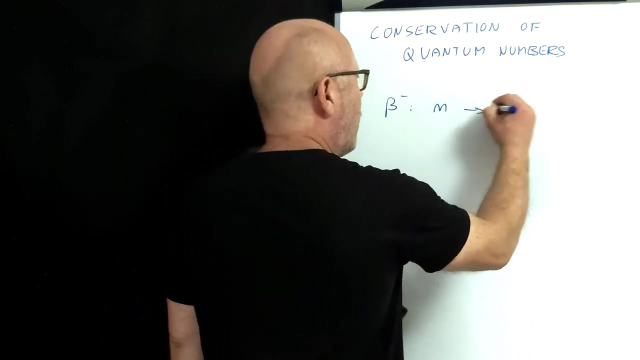 this idea to predict if some reactions in particle physics are possible or not. Let's start with this possible Beta decay. So you know that in beta decay let's consider beta minus, right, That's a neutron that becomes a proton plus an electron plus an antineutrino of the electron. A neutron is 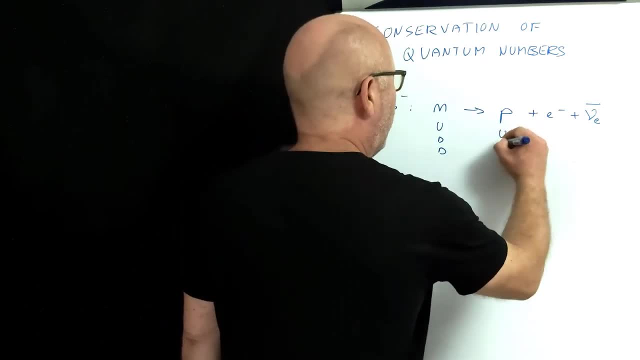 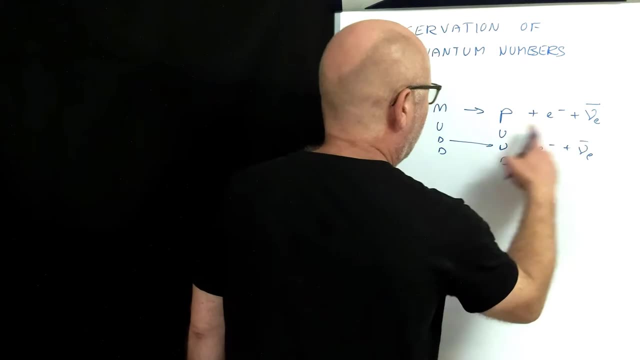 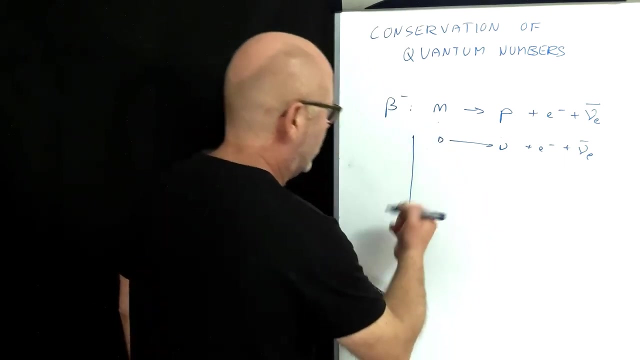 up, down down, And a proton is up up down. So actually this is a down becoming an up plus an electron, plus an antineutrino of the electron. Remove these Now. to check if this is possible, I suggest to my students to just write down the quantum numbers Q, B, L and S. 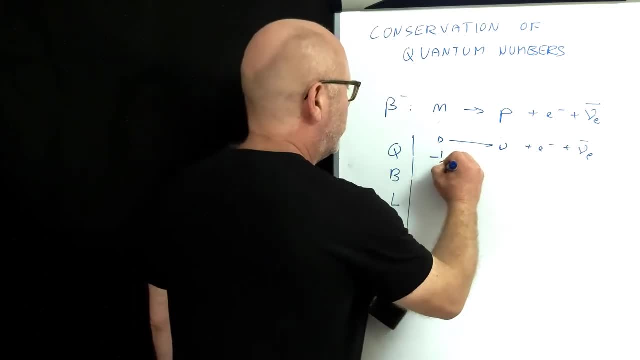 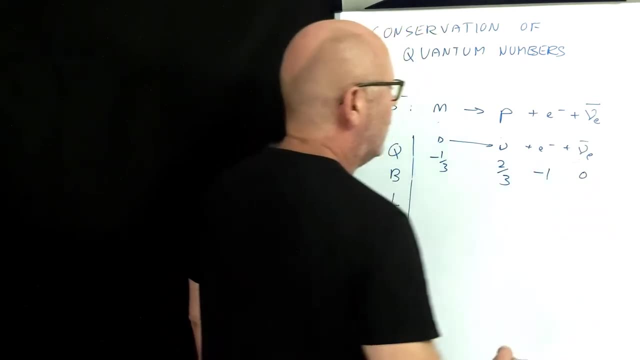 For the down quark, we know that the charge is minus one-third. For the up quark it's plus two-thirds, For the electron it's minus one And the antineutrino is zero. Minus one-third is equal to two-thirds minus one. 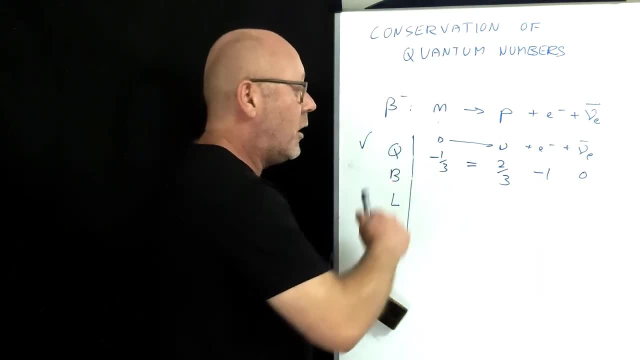 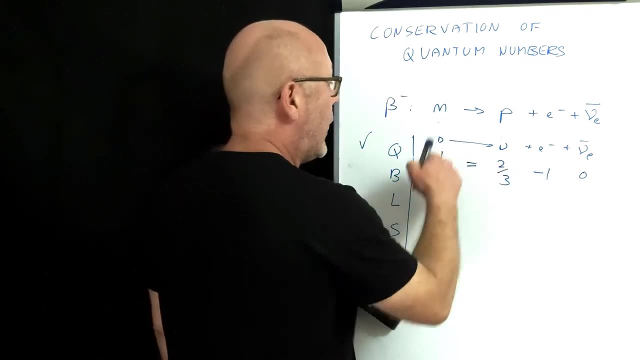 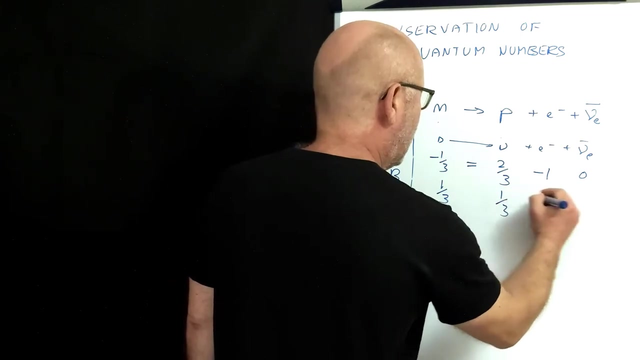 Check. The conservation of charge is respected by this reaction. Let's try the baryon number. The neutron is a baryon. Yeah, I could use also the down quark. Let's use this. one Down quark has got a baryon number of one-third. the up quark of one-third the electron zero antineutrino of the. 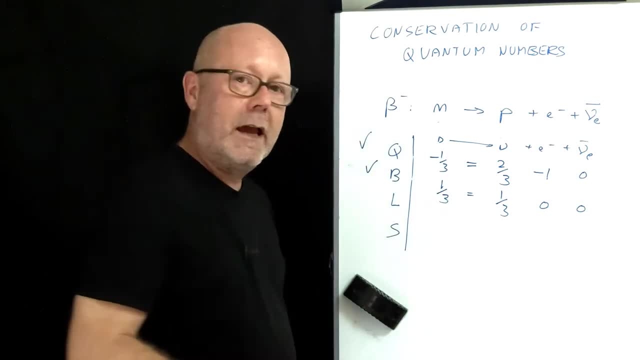 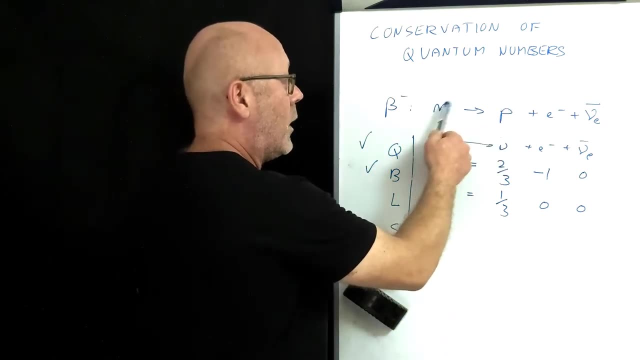 electron zero. It's equal The baryon number. check This reaction respects the conservation of the baryon number. I could have used neutrons and protons one and one, zero, zero. It would have worked too. 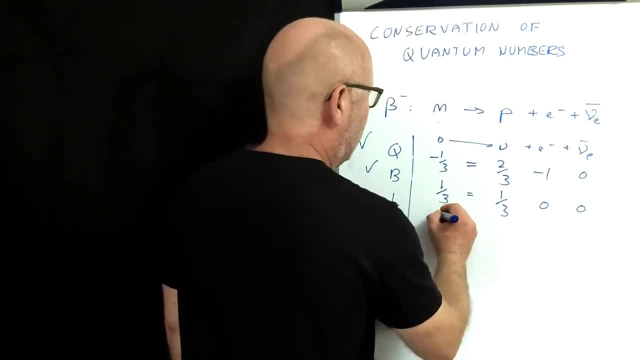 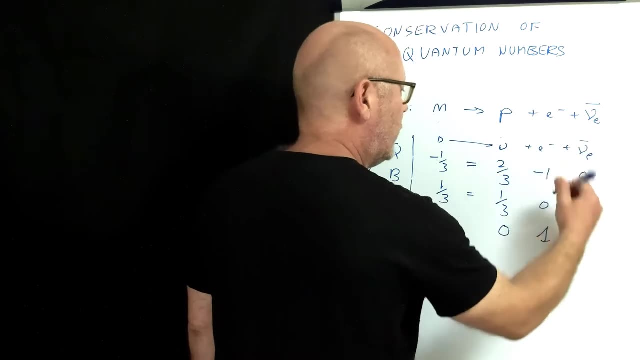 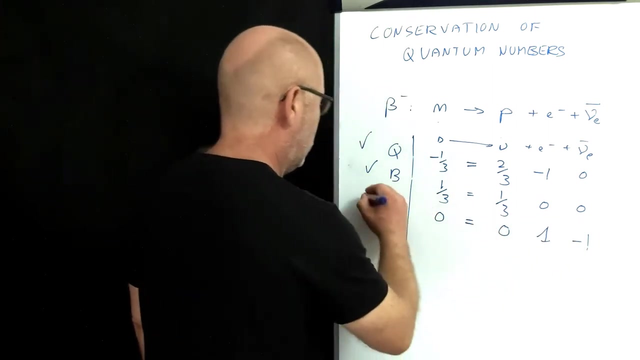 Lepton number. So down it's a quark, so it doesn't have a lepton number, neither does the up. The electron is actually a lepton, so plus one, and the antineutrino of the electron is an anti-lepton, so minus one Zero equals zero one, minus one zero, So check. 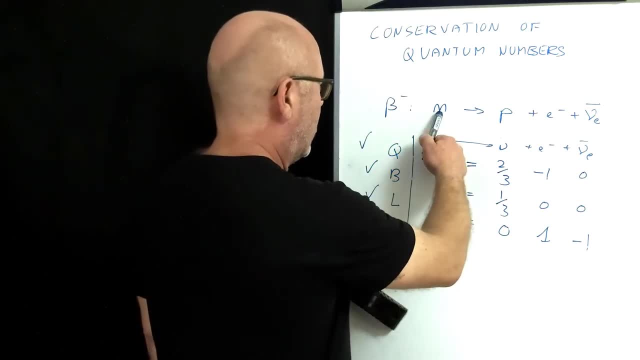 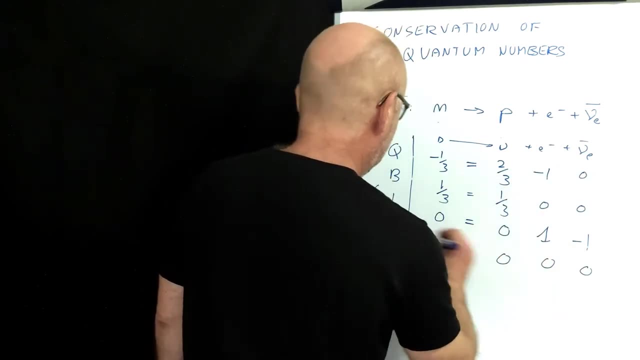 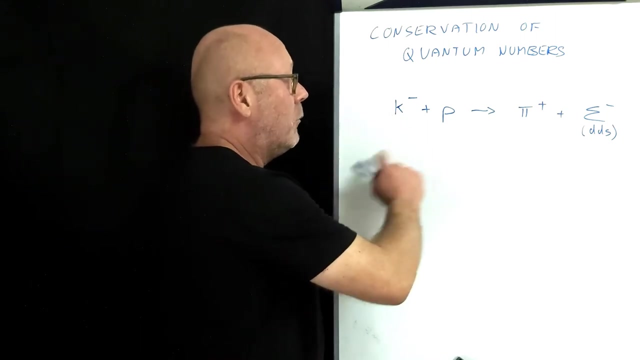 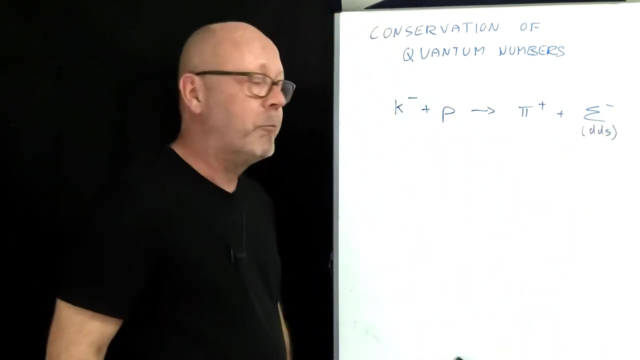 Let's check strangeness now. Are these strange? No, Are these quarks? No, Check, This reaction is possible. In this reaction we have a negative count plus a proton that transform into a positive pion, plus a sigma minus, which is a baryon. 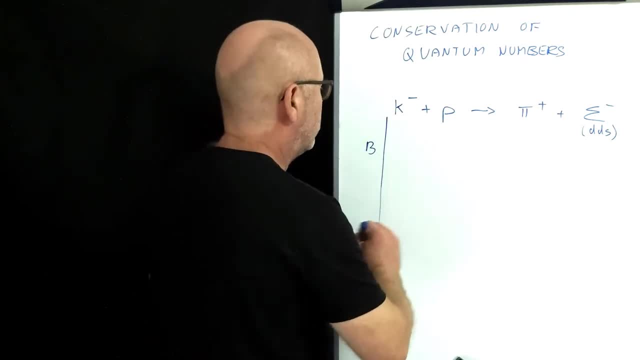 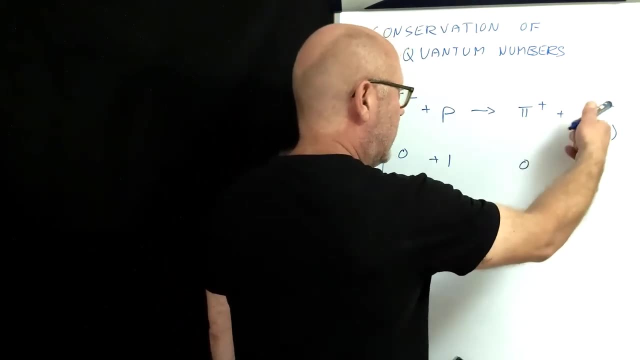 So let's start. Baryon number: Baryon number: This is not a baryon. The proton is a baryon. This is not a baryon. That's a baryon. So we got one equals one Check. 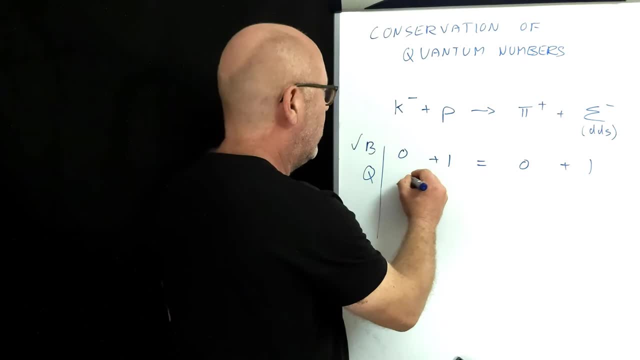 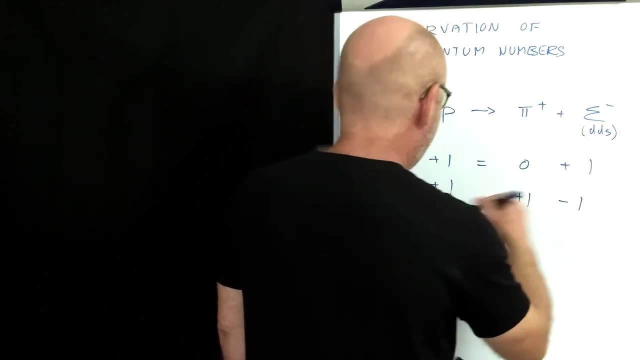 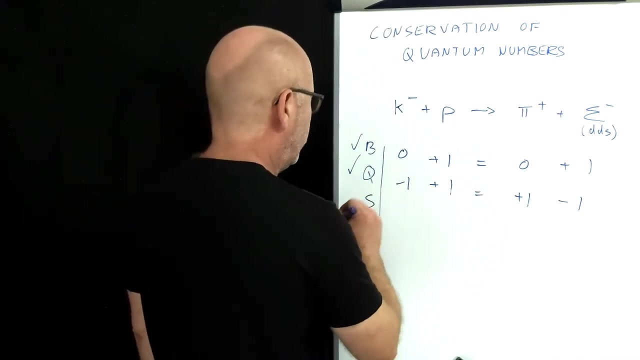 Charge: Negative charge minus one. Proton has got a positive charge, The pion plus one, The sigma minus negative, one Minus one plus one is equal to plus one negative one. So check, Let's check the strangeness. Well, chi minus it must be. 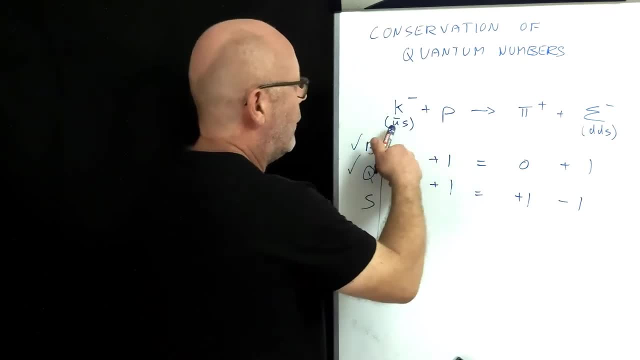 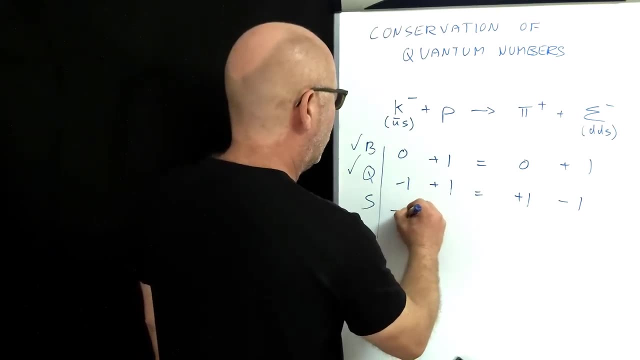 let me think an anti-up and a strange: Minus two-thirds, minus one-third is minus one. So it has some strange. So it has some strangeness. So it's going to be minus one. The proton has no strangeness. 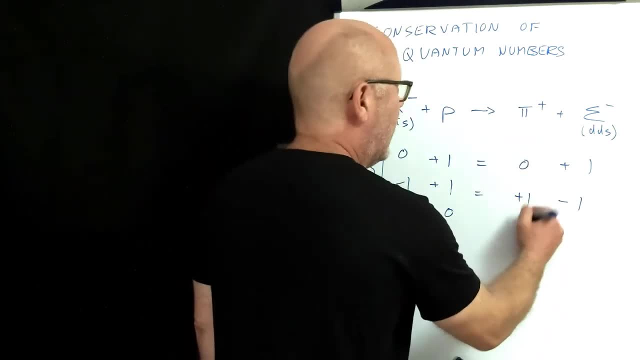 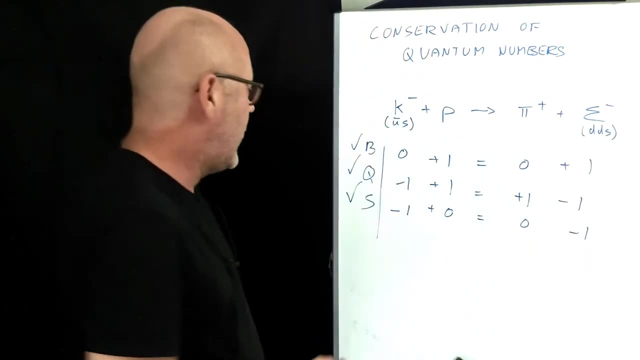 The pion is only made of up and down, So no strangeness. And the sigma has got a strange quark. So minus one Check. And finally, let's look at the lepton number. Well, we don't have to think. 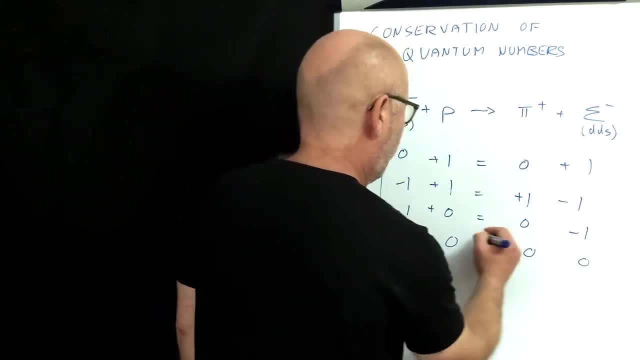 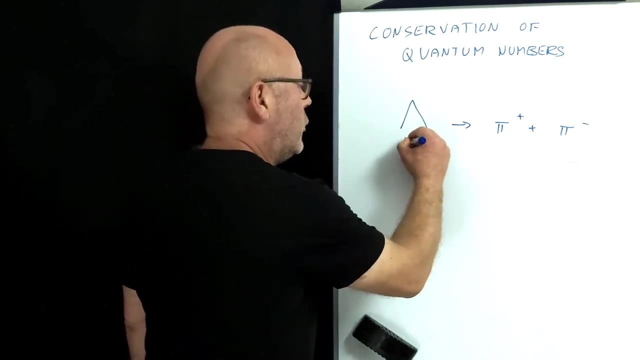 too much because there's no leptons involved. So zero equals zero. Check: This reaction is possible. In that case we have a lambda which is Udl And, yes, transforming into a pion positive plus a pion negative. 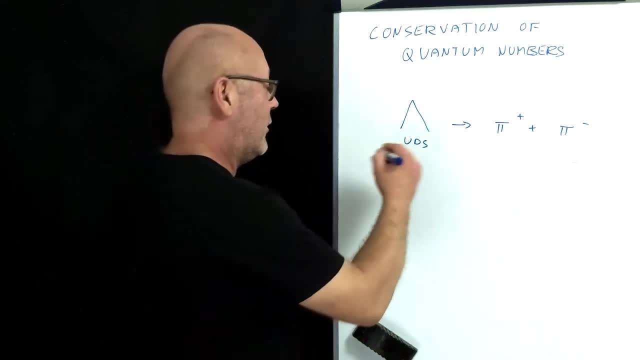 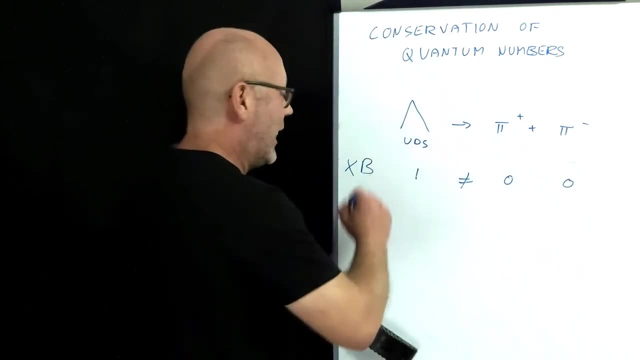 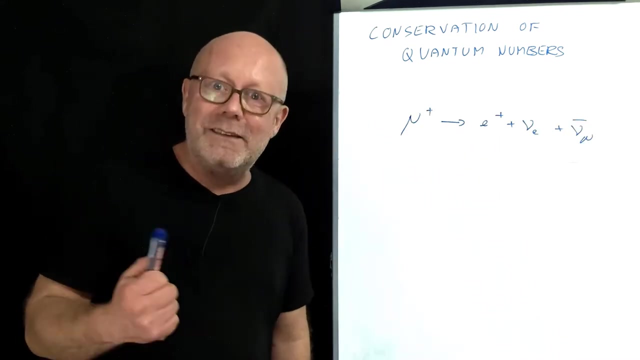 I can see immediately that won't work. That won't be possible because when I look at the baryon number, this is a baryon and these are mesons. So no baryon number, Not check. I don't need to continue further. I know this is not possible. Let's play with. 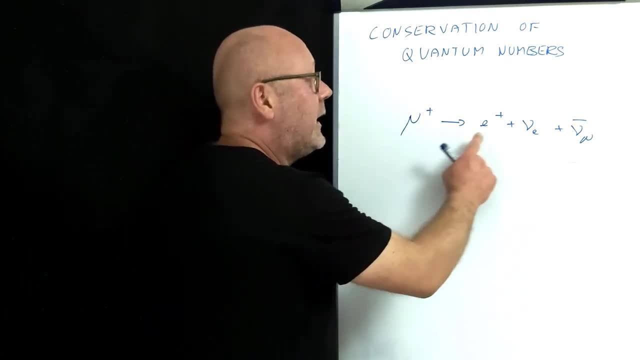 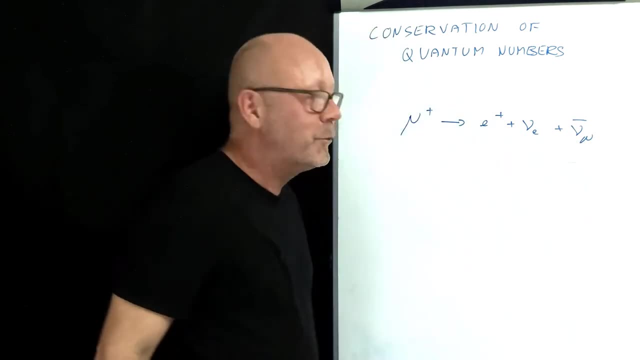 leptons. now We have this antimuon that decays into an antielectron plus electronic neutrino And a muonic antineutrino. Baryon number: Well, we know it's going to be zero and zero. 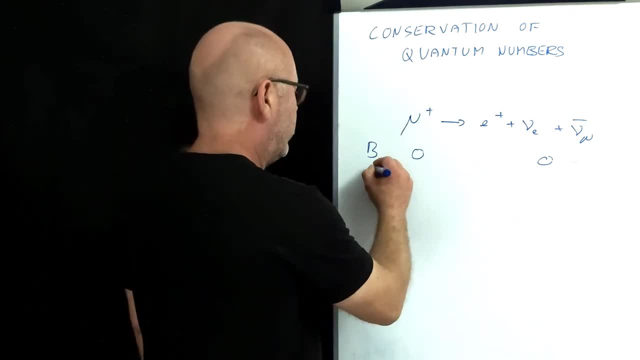 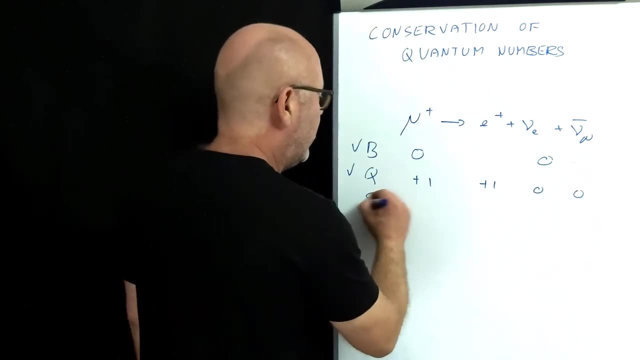 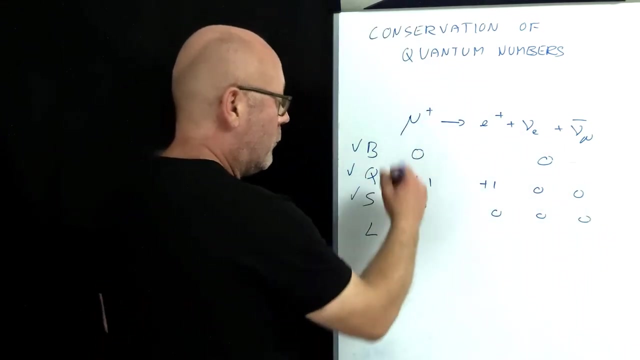 Because there's no baryon involved. Charge Plus one Plus one, Zero, Zero. Check Strangeness: There's no quarks involved, So there won't be any strange Lepton number Minus one for the antimuron. 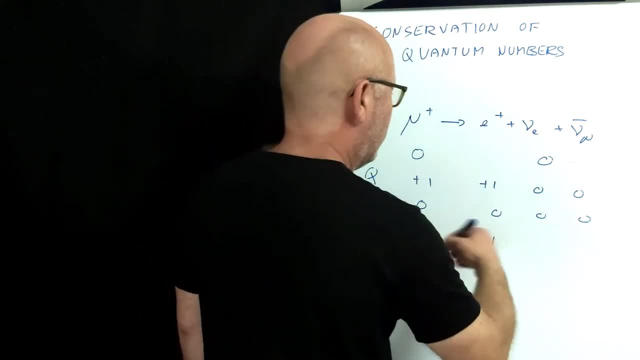 Minus one for the antielectron, Minus one for the antielectron, Minus one for the antimuon, Minus one for the antimuron, Minus one for the antielectron. plus 1 for the electronic neutrino, minus 1 for the muonic antineutrino. 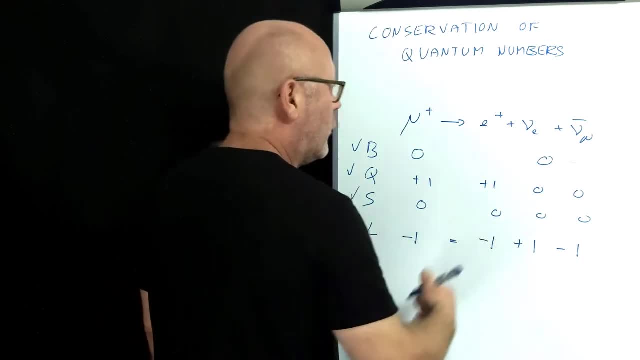 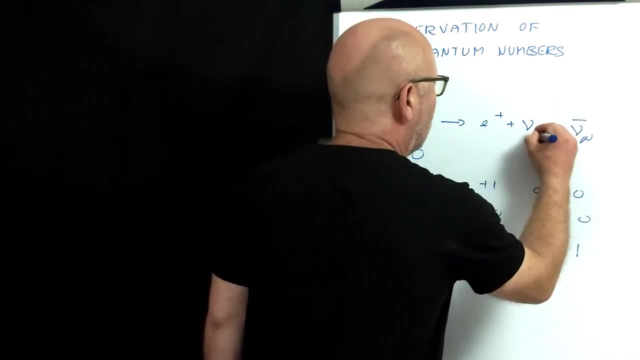 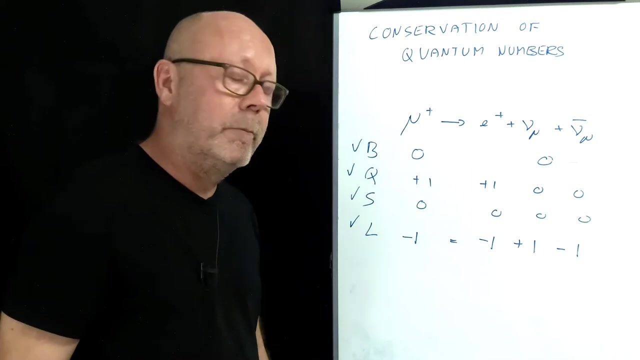 So it works right. We've got minus 1 equals minus 1.. But be careful, because if I did this, for example, it would work too right. The neutrino of the muon would still give you a lepton number of plus 1.. 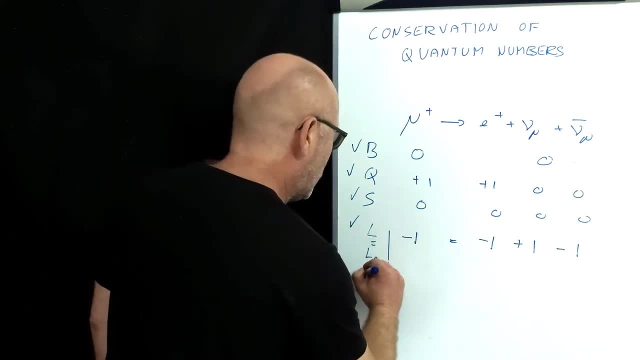 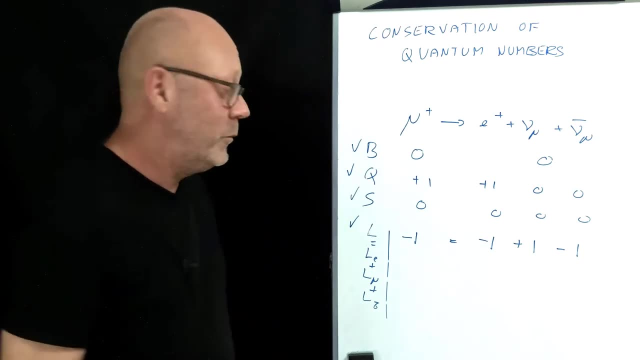 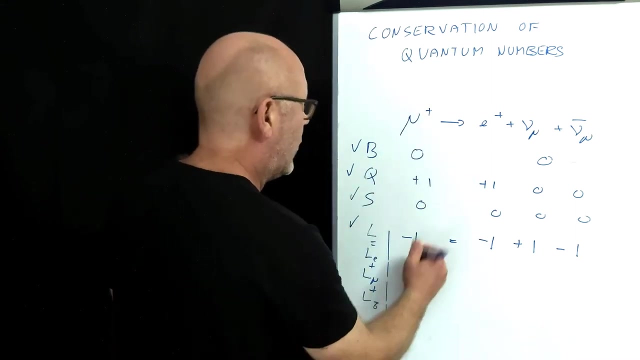 L is actually the electronic lepton number plus the muonic lepton number, plus the tauic lepton number, And all these components need to be conserved also. So for example, let's consider the electronic lepton number. This is not an electron, so 0.. This is a positron, so minus 1.. 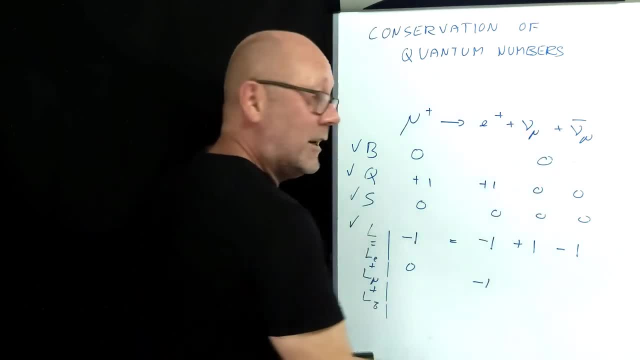 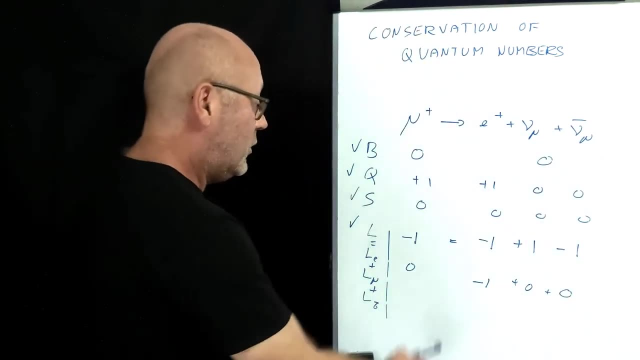 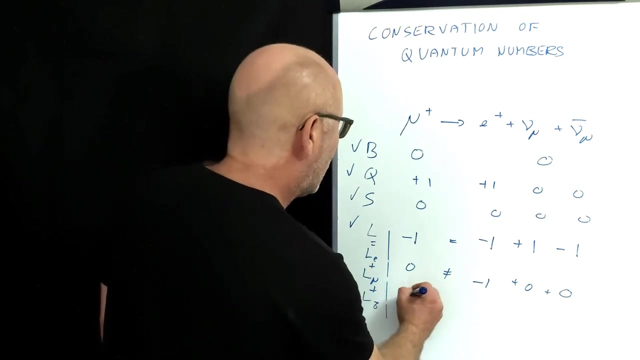 This. so the muonic neutrino is not electronic, so it's 0. And this would be 0 too, Nothing to do with electrons. So you see, that's not conserved. If I do the muonic lepton number, that would be minus 1, that would be 0, that would be plus 1, that would be minus 1.. 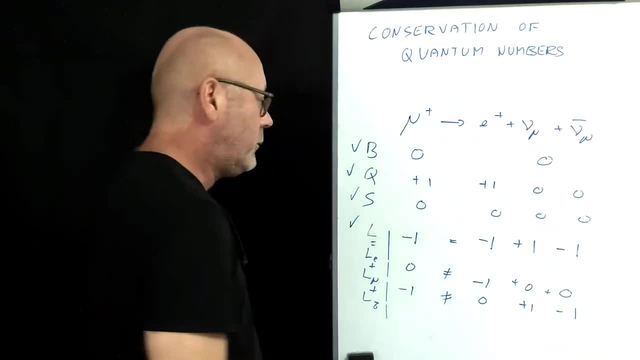 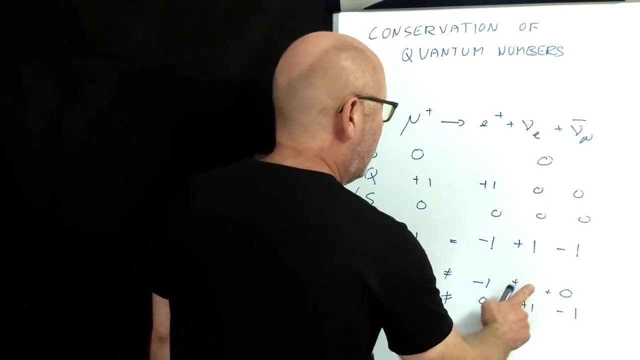 Again, you have minus 1 equals 0, so it's not conserved. In order for this to be conserved, that needs to be an electronic neutrino Like this. you would have plus 1 here and here you'd have 0. 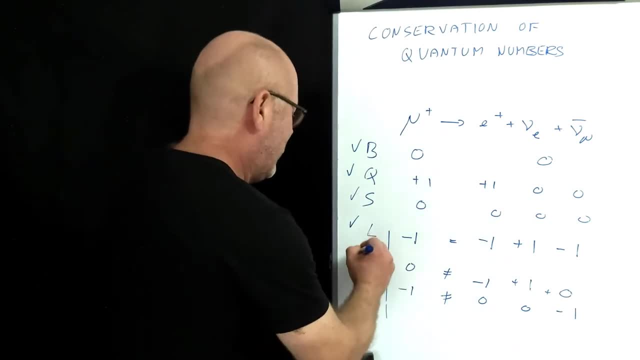 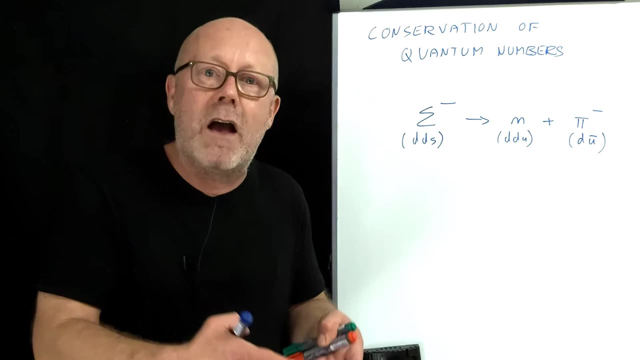 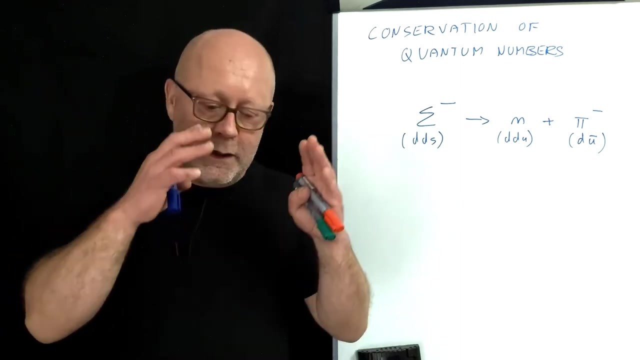 And then you could check. There is one exception, though, that you need to know within the scope of a high school program in physics. We've just seen here that all the quantum numbers need to be conserved if we want to verify that a reaction is possible. 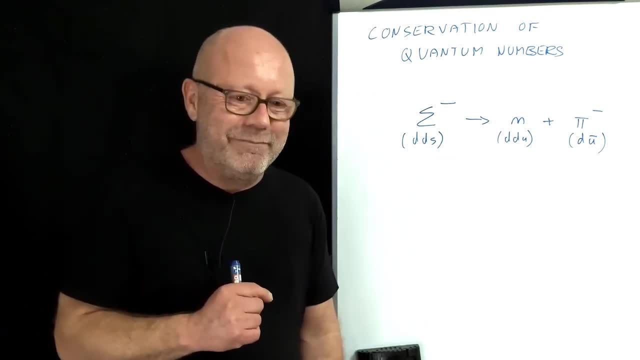 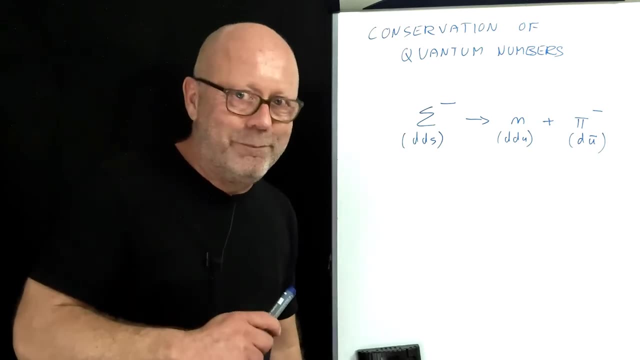 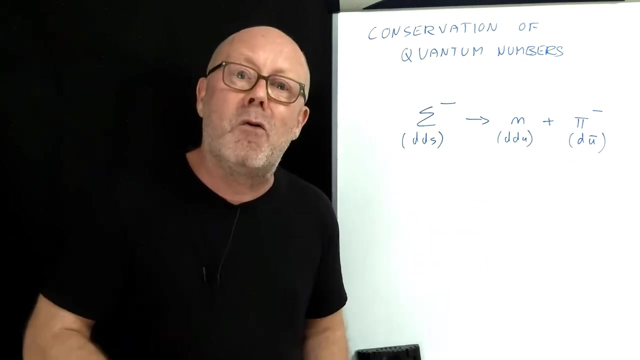 There's one exception: If strangeness is not conserved, you would say, OK, this reaction is not possible. It's not always true. If it is the weak force which is involved in the reaction, then it is acceptable to consider strangeness as not conserved. 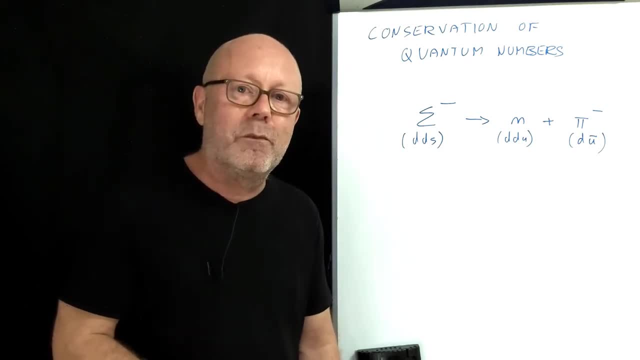 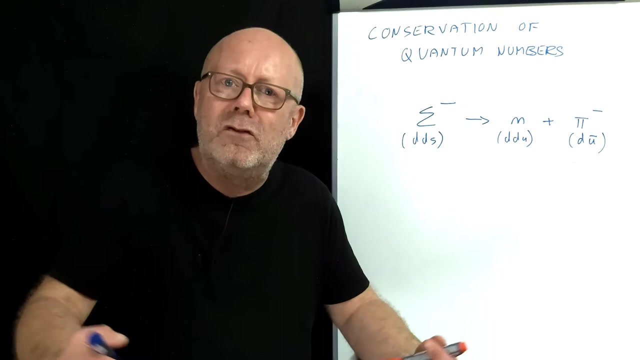 The reaction will still be possible. The reason for this is that the consequence of the action of the weak force is that one quark can change into another. So if, in the reaction, the weak force changes a strange quark into something else, like a down or an up, of course strangeness will change. 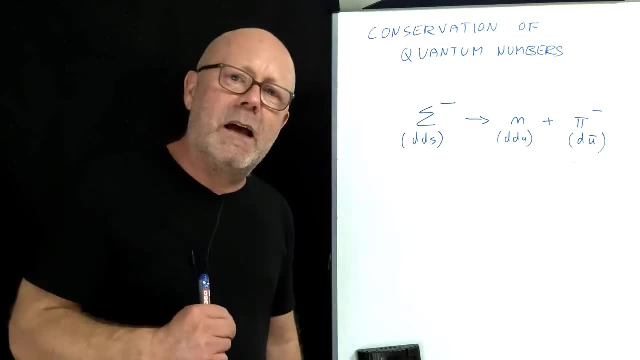 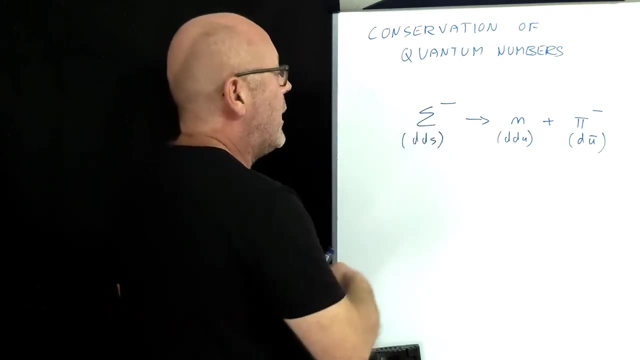 And the reaction is still possible. To give you an example, we have a negative sigma that transforms into a neutron and a negative pion. The negative sigma is made of down, down and strange. The neutrons: down, down and up. 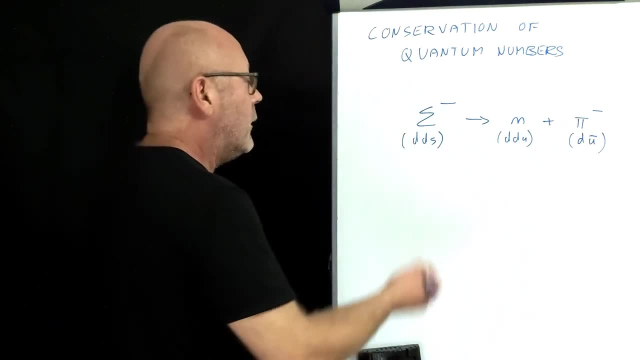 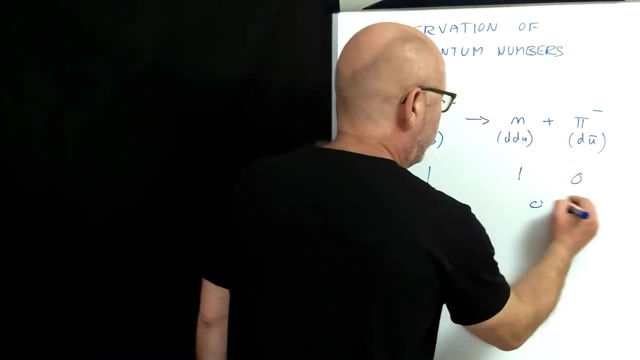 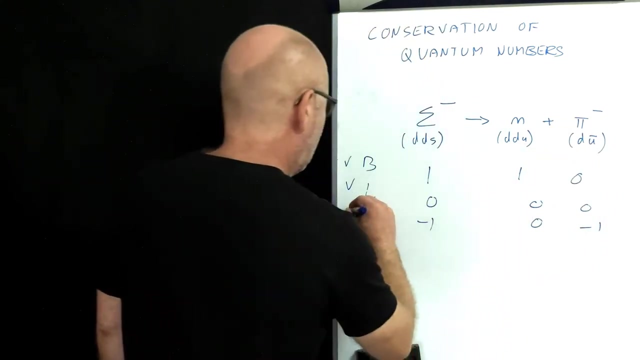 And the negative pion down and anti-up. Baryon number 1,, 1,, 0 conserved. Leptron number 0 everywhere. Charge Negative: 1. Negative 1. Neutron is neutral, so 0 conserved. 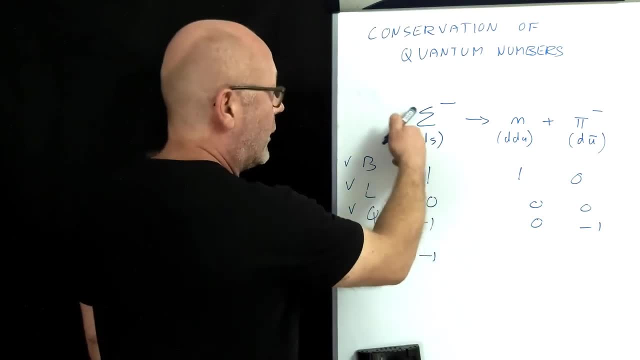 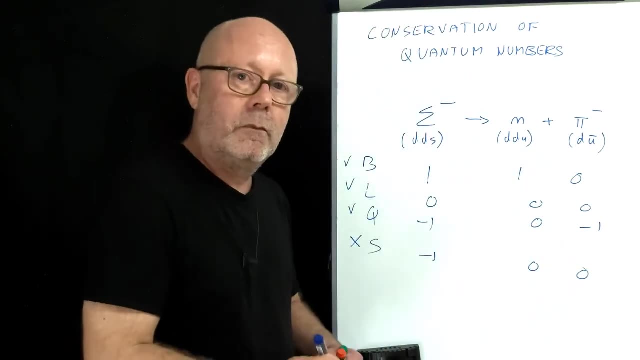 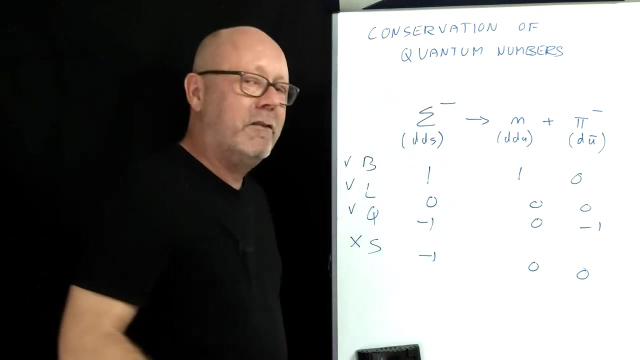 Strangeness: Negative 1 because we have a strange quark in the sigma, But we don't have any strangeness here, So strangeness is not conserved. However, in the text you should have information about what force is involved. 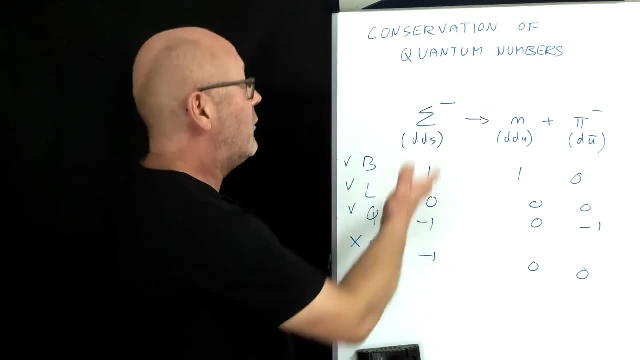 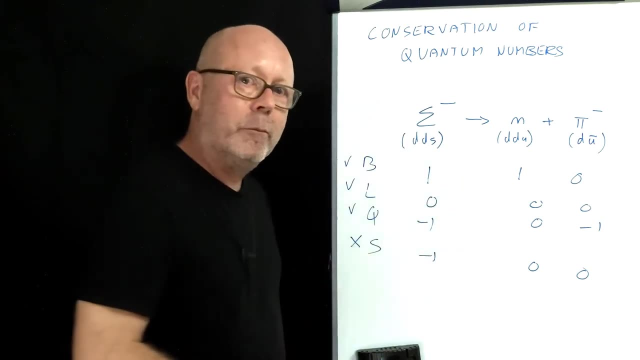 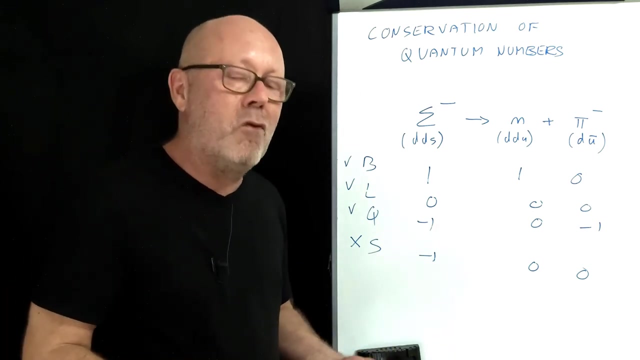 If they say it is a strong force that creates this reaction, then you know it's not possible. But if the text says it is a weak force which is involved, then the reaction is still possible, Got it? It might also inform you in the text that the weak force is involved in a hidden manner. 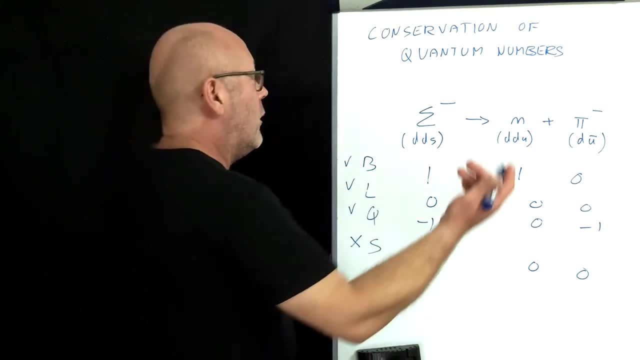 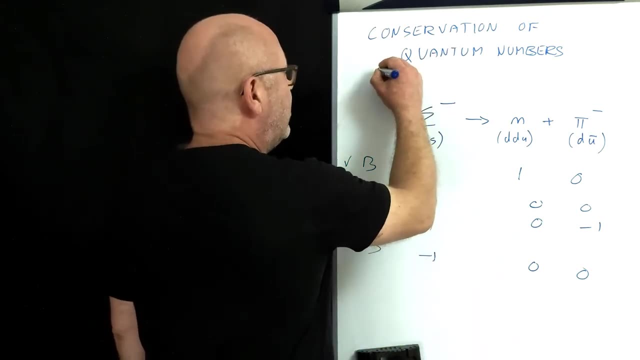 They will give you the rate of reaction, meaning they will tell you the half-life of the reaction, say how long it takes for half of the sample to react. If they say that it goes very fast, something like 10 to the minus 28 seconds. 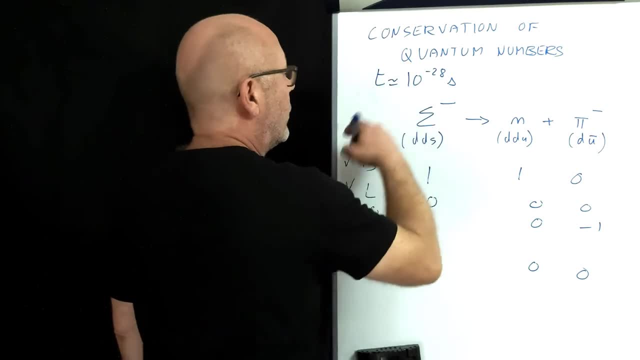 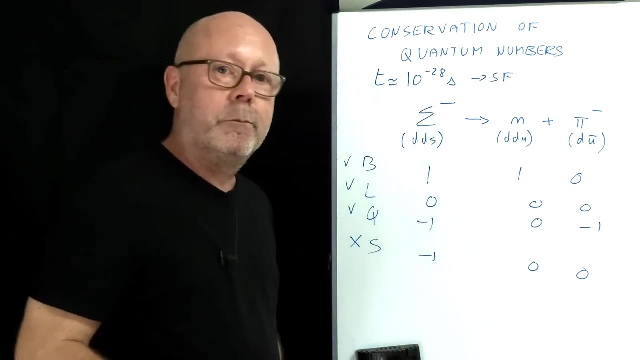 you know, it's the strong force which is involved. So if the reaction is fast, this is not possible. On the other hand, if they tell you that the reaction rate is something like 10 to the minus 11 seconds in this range here, then it would be the weak force which is involved.